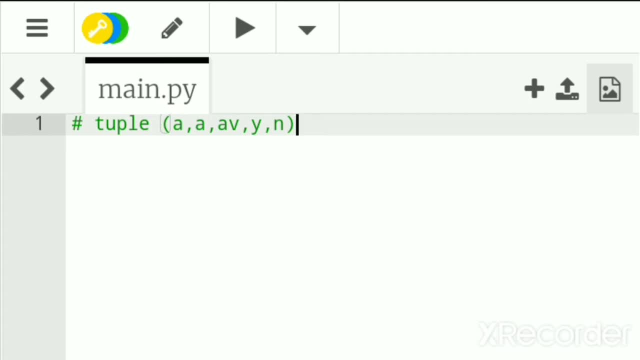 between the two. so the two are constructed in the same, in the same manner, and we can have index on them, you can make slice in on them and we can make many, many operations on the 2. but there is just one differences between the two is that tuples are unchangeable and 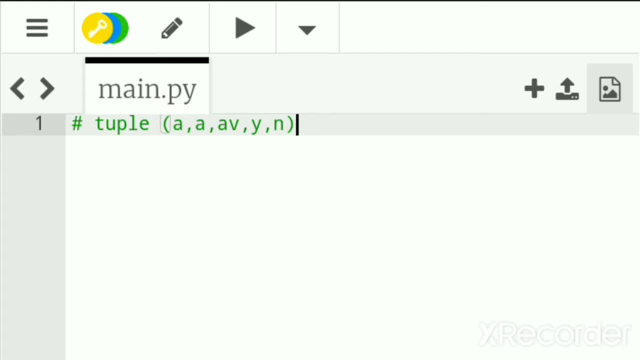 ordered sequences. what it means. That means that ordered, that each elements in a tuple, an order, and the second, it is unchangeable, which means once the tuple has created, we cannot change its elements, we cannot add elements and we cannot remove any elements of this tuple. this is the big difference between or 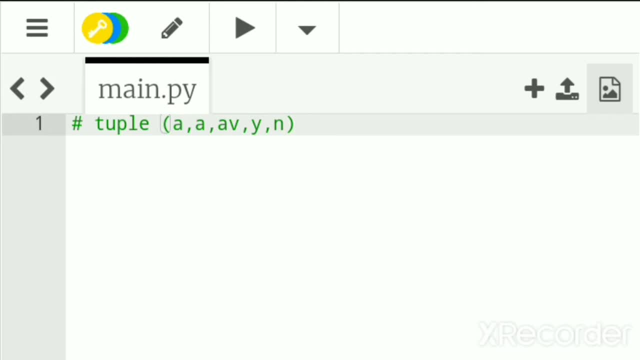 differences between these two objects and the two sequences in Python. so we see some examples. for example, if we want to create a tuple, of course we can do this with the round brackets, for example with integers. so it is the same thing as in a list, so we can print. 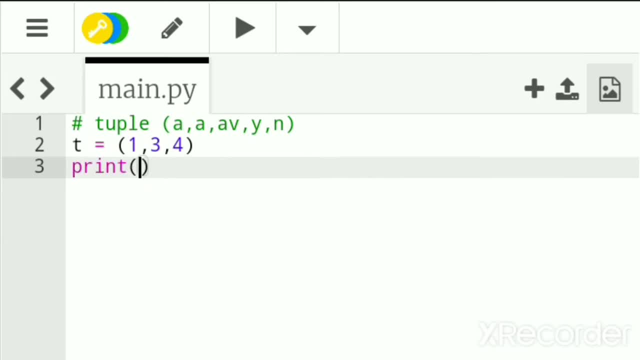 print this tuple without any problem. so, as you see, and we can also add strings. so banana, no problem. we can also add boolean values, no problem. so all this are accepted just like this. so it is there and they are. they are accepted in tuples. good, we can also just indicate the elements that we want to print by. 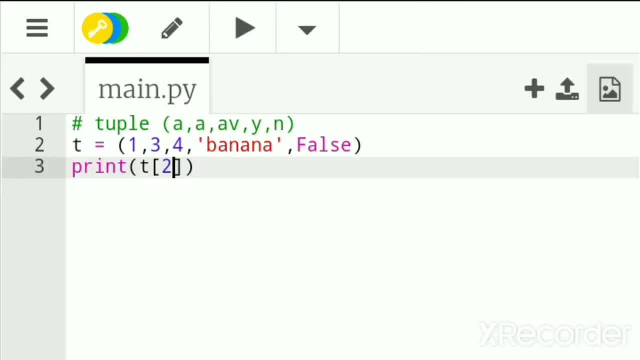 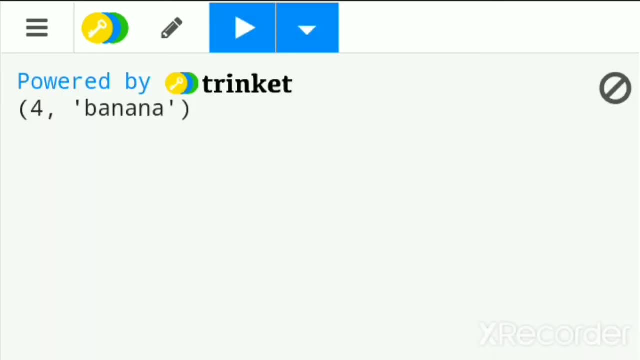 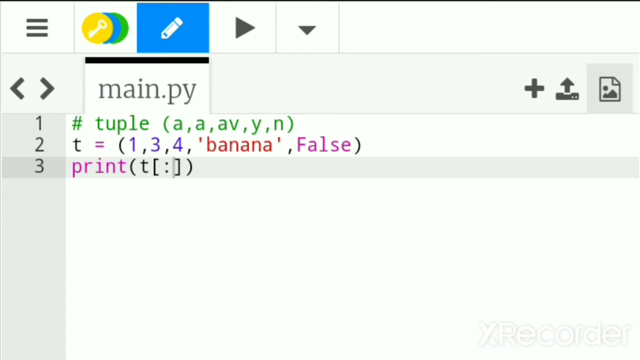 indexations. we can also make some slicing, for example. so we can do this. and of course we can do all what we have seen in the last session on the tuples on the list- good, but of course, as I said, we cannot write, for example, we cannot change. 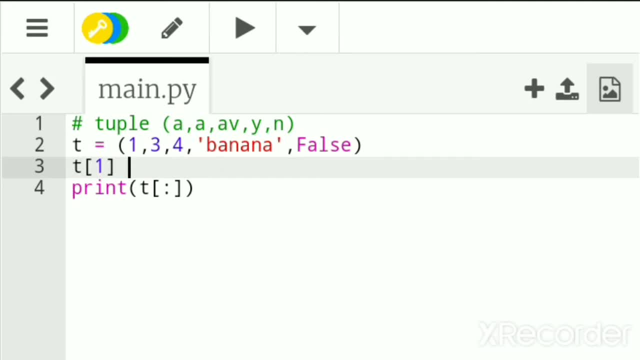 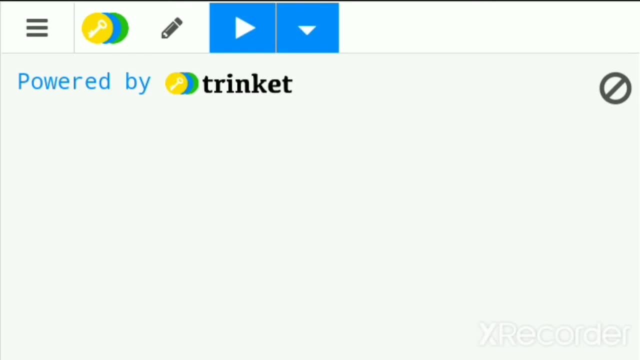 we cannot write, for example, we cannot change, we cannot change. we cannot change any elements. for example, if we try to change the second elements, for example by this number, this, there is an error. so here we the right type error. tuple does not support item assignments, so we cannot change the second, the second. 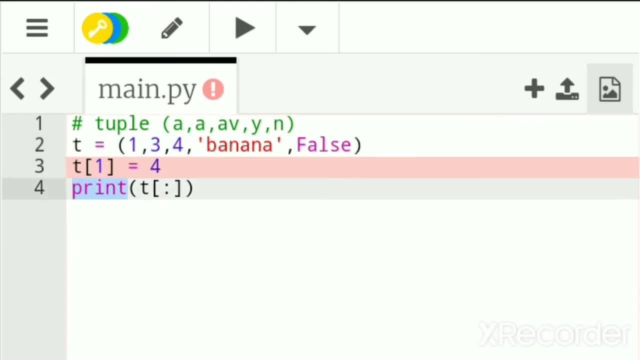 element. so this writing is this one, it is typically this one. it is typically wrong. so we can not write this. so we cannot move or remove anything from this wrong. so we can not write this. so we can not move or remove anything from this tuple, for example, if we're trying to write this, so there is another problem. so some object incident. 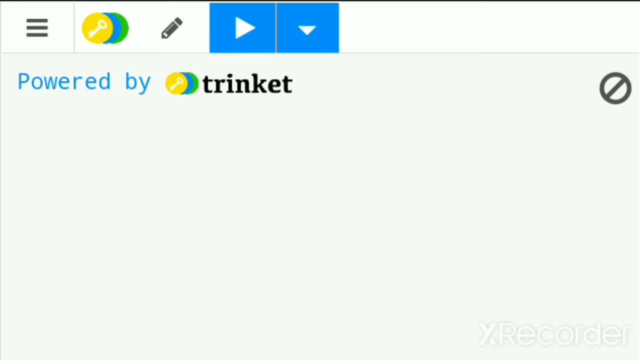 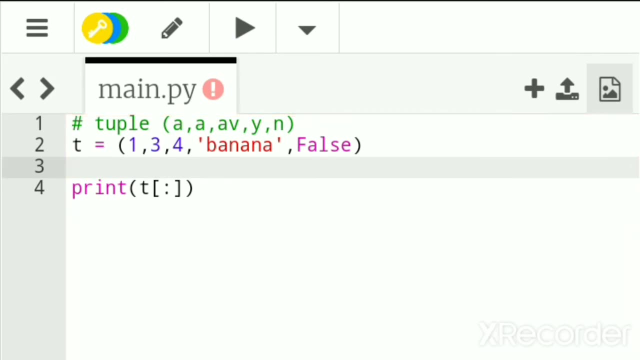 our object does not support item deletion, so it is in the limit setting now. so, for example, if we would likeoud to, impossible, good. so there is another example. what if we have just, uh, if we have a tuple that just have one item, for example? so can we just write it like that? so if we try to to to print it, 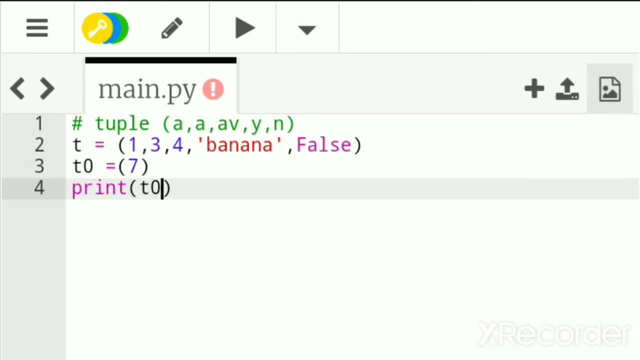 so t zero, so we have seven, but the seven it is not a tuple. so if we try to see the type type of this, this object, it is integer, it is an integer, it is not a tuple. but if we want it to be a tuple, what can we do? just, we can just.